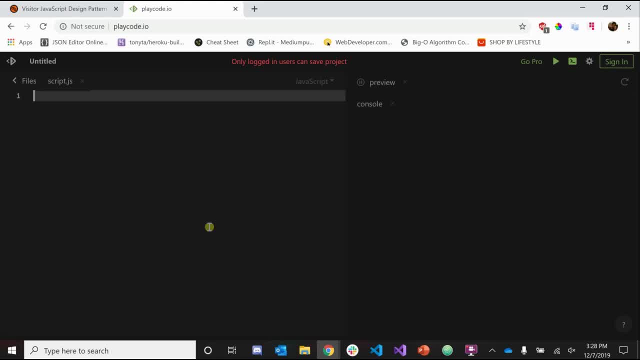 employee class. The employee will have a name and a salary and we're going to need to be able to get and set the salary. so we're going to have a get salary and a set salary method And after we get all that working, we're going to extend the 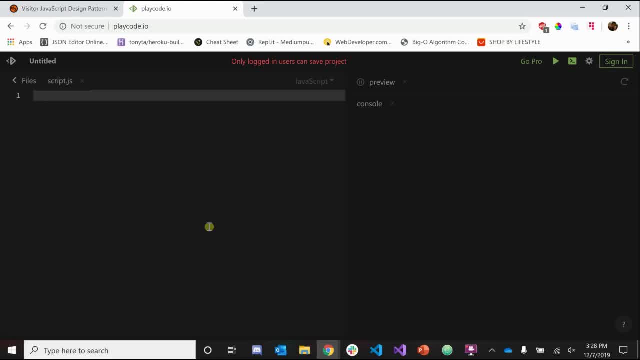 functionality of our employee class using the visitor pattern. So let's go ahead and jump into it. So let's create our function. employee and employees are going to have names and salaries, So we're going to set thisname equals name and thissalary equals salary. 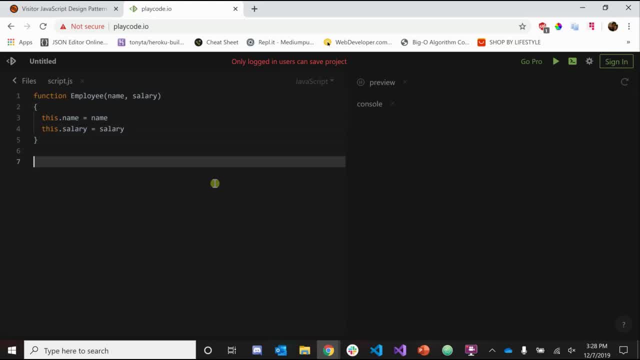 Okay, we have our properties. now we need to have create our methods. so we're going to go down here and say employeeprototype and we're going to have our get salary method. This is just going to return thissalary. Okay, now we need our set salary method. 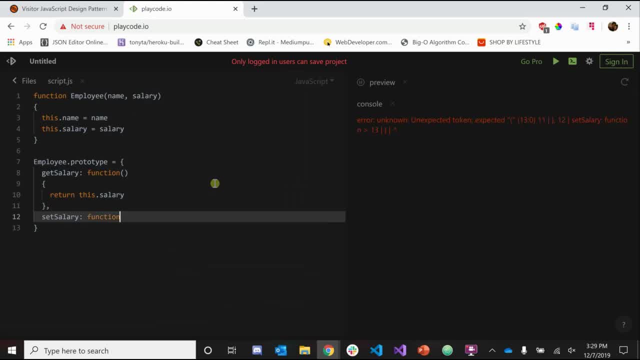 We're going to say set salary function. We're going to take in a salary, We're going to name it sal and we're going to say thissalary equals sal. Okay, and we also need one more method, The accept method that takes in a visitor function. 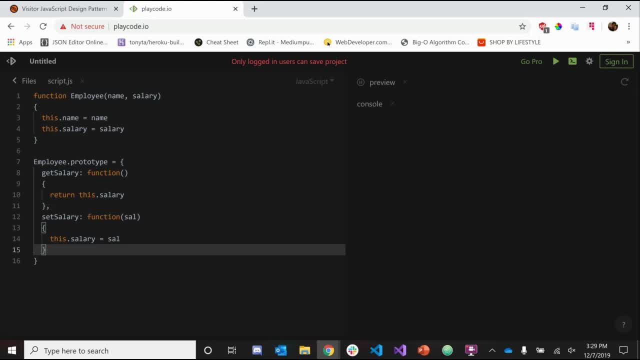 and gives the visitor function access to this employee object so that it can manipulate and access its properties. So let's create that. So let's say accept function and this is going to be a visitor function and we're just going to say, we're just going to call this visitor function, passing in this, which 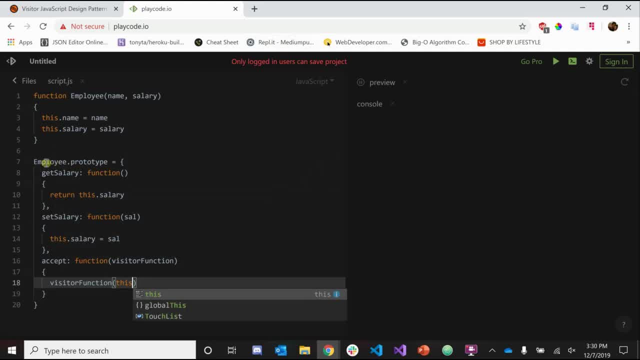 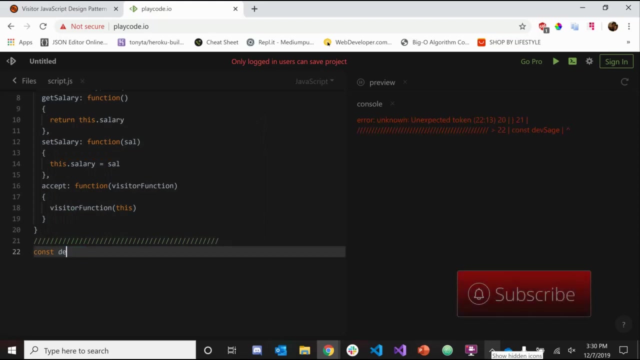 is a reference to this employee. Alright, we are done with our employee class, so we're going to go down here. We're going to just create like a separator here. So let's create a new employee. So let's say const dev sage. Let's say dev sage equals new employee. 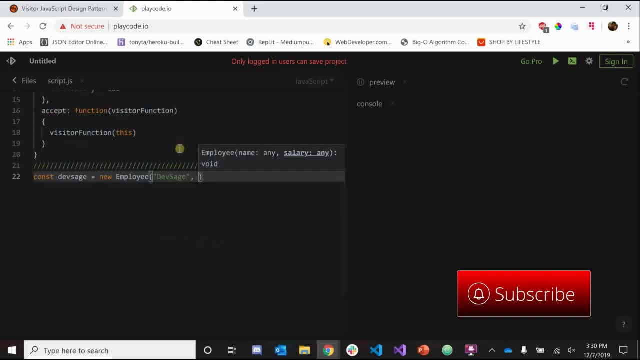 dev sage for the name, and let's say my salary is now ten thousand. Let's say I make ten thousand dollars, Okay, so let's print out my salary. So let's say console log, dev sage, dot get salary. All right, ten thousand, Okay, cool. so let's try to extend the. 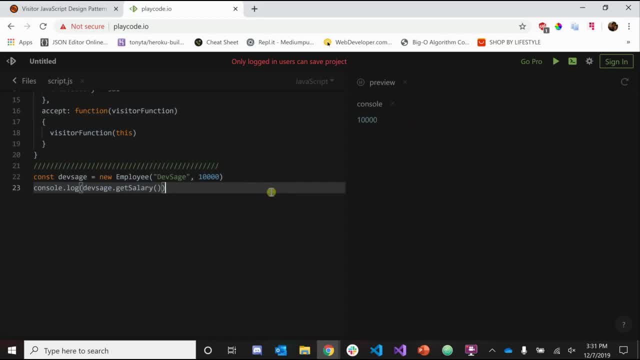 functionality of our employee class. Let's try to modify a little bit. So let's create our visitor function, and our visitor function is going to actually give me a raise, So we're going to modify it by a little bit. So when I click this angry button, I'll preempt my salary function by исc. 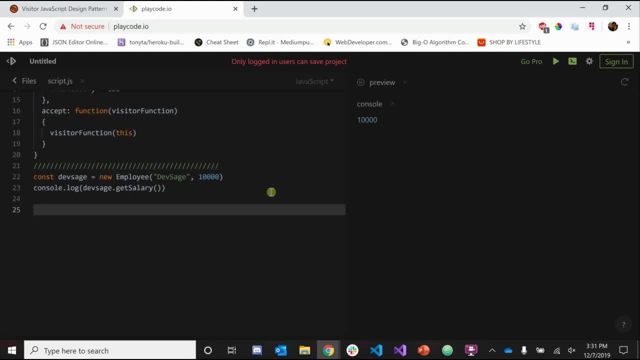 our salary to return twice my current salary. so let's create that function. so it's a function, extra salary- and we're going to take in an employee and we're going to say: EMP- employee dot set salary, EMP dot get salary times two. so extra salary is our visitor function. it's going to take in an employee and it's. 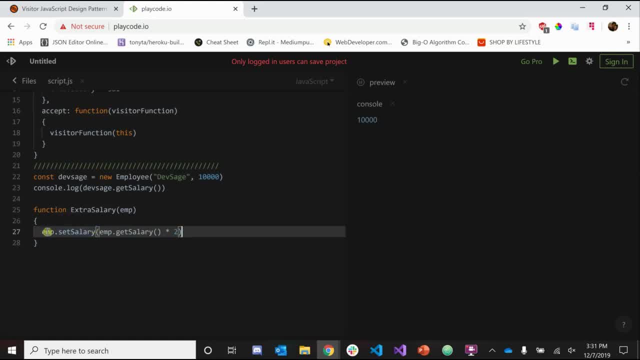 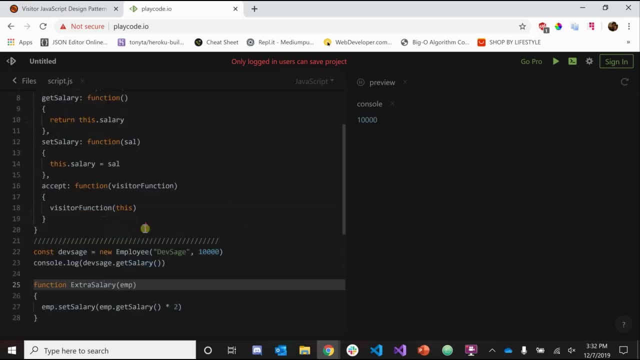 going to call the set salary method on this employee, setting my salary to be twice my current salary. ok, cool, but how is this actually going to work? I can't actually. we're not going to change our employee class. how is my visitor function going to know anything? 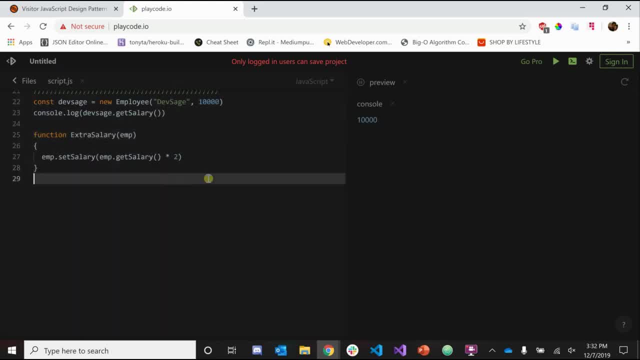 about my employee. so we're going to use that except method we made earlier. so we're going to say dev sage, dot except, and we're going to pass in extra salary. we're not going to call it, we're just going to pass in the name extra salary. 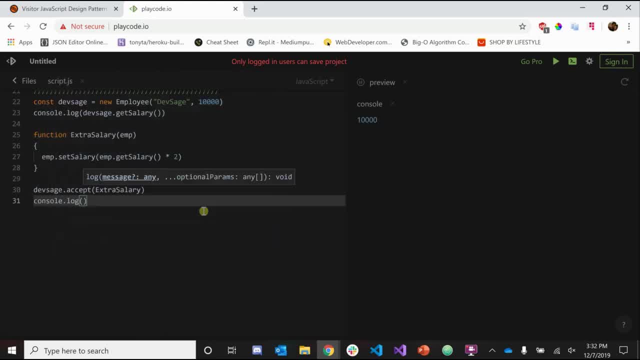 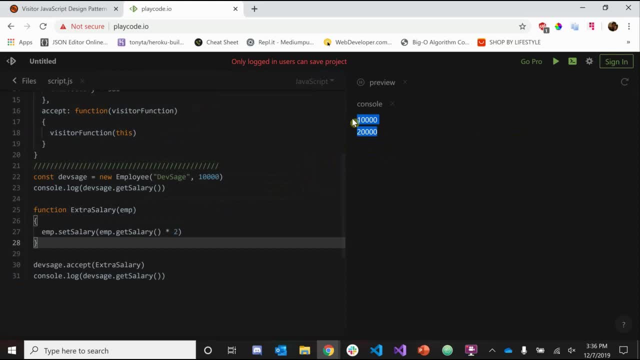 you and let's try printing out my salary again. so dev sage dot, get salary and look at that. 10,000 and 20,000. our 10,000 comes from our first call to get salary right after we create our employee and our 20,000 comes from our